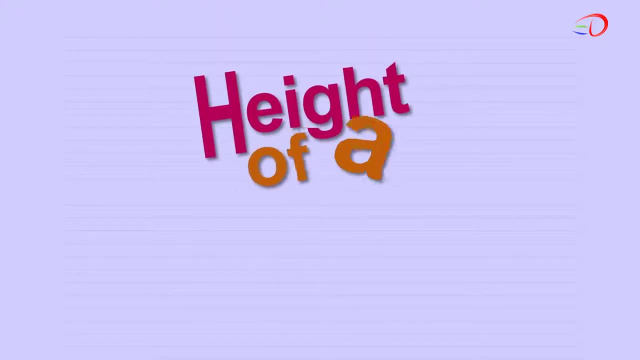 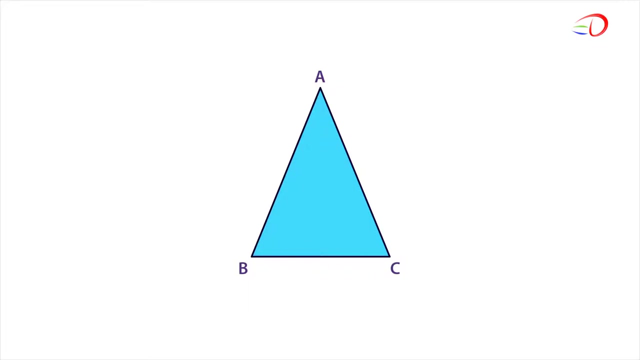 Do you know how to find the height of a triangle? Let's look at the triangle ABC. Let's take BC as the base To find the height. look for the vertex opposite the base, So A is the vertex. Now draw a perpendicular line from vertex A to the base BC to form a right angle. 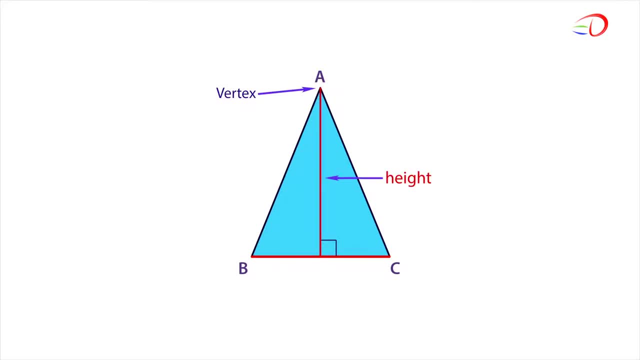 So when BC is the base, this is the height. Let's look at triangle DEF. Take EF as the base. Where is the vertex opposite the base D? From vertex D draw a line to the base. It doesn't meet the base EF. 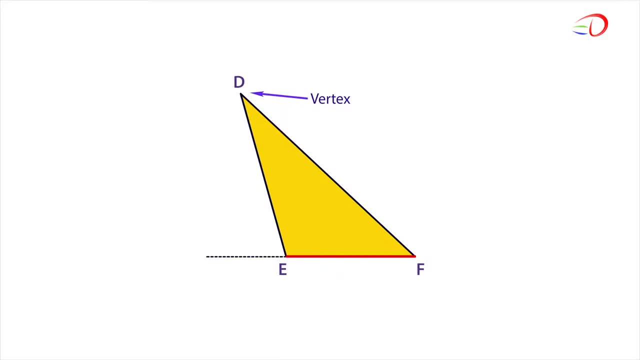 What should we do? Extend a line from the base EF. Now draw a perpendicular line from vertex D to the extended line to form a right angle. So when EF is the base, this is the height. Let's look at triangle XYZ. 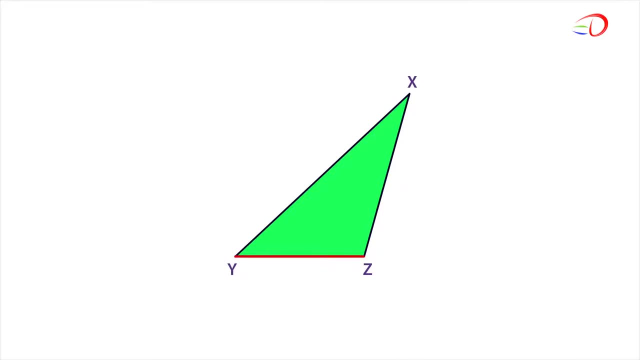 Take YZ as the base. Where is the vertex opposite the base X? From vertex X. draw a line to the base. It doesn't meet the base YZ. What should we do? Extend a line from the base YZ. 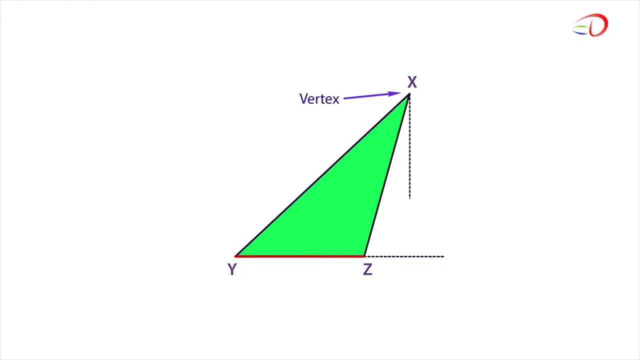 Now draw a perpendicular line from vertex X to the extended line to form a right angle. So when YZ is the base, this is the height. Now that you know how to find the height of a triangle, you can calculate the area of any triangle. Now take YZ as the base and calculate the area of the triangle. So when YZ is the base, what should you do? Extend a line from the base. draw a straight line from vertex X to the extended line to form a right angle. If you don't have the right angle, then you can't say that you can't have the perfect level. So what should we use to calculate this angle? We can also use the Law of Among the Vertical Mathematics. Here is our diagram.